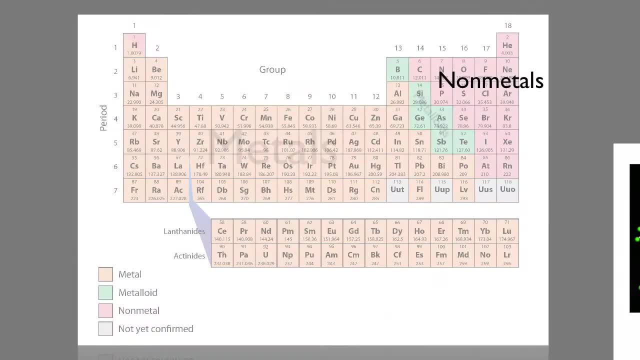 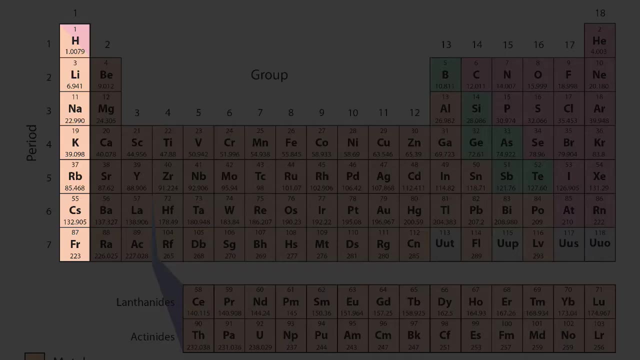 of nanotechnology. The metalloids only sort of conduct electricity, which is to say they're semiconductors. The most famous semiconductor of them all is silicon. A vertical column in the periodic table is called an atomic group or sometimes an atomic family, Elements within the 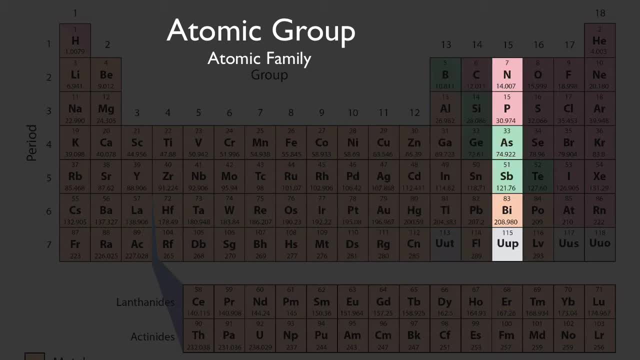 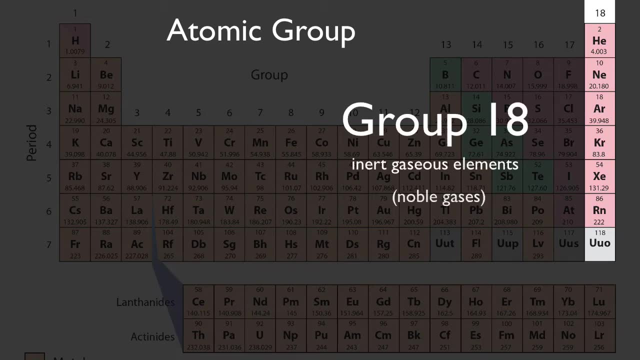 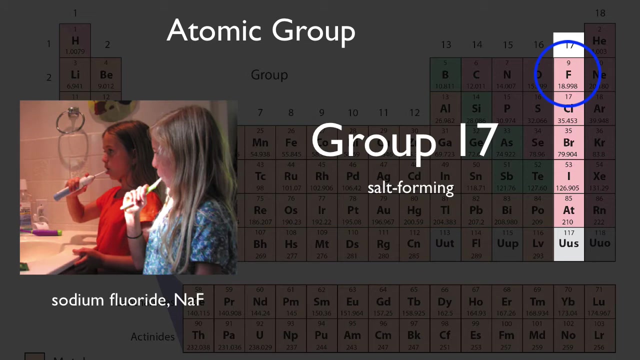 same group or family share similar physical and chemical properties. All the group 18 elements. for example, they're inert gases. We call these the noble gases. The group 17 elements: all tend to form salts, such as sodium fluoride, which in small amounts is good for your teeth, or sodium. 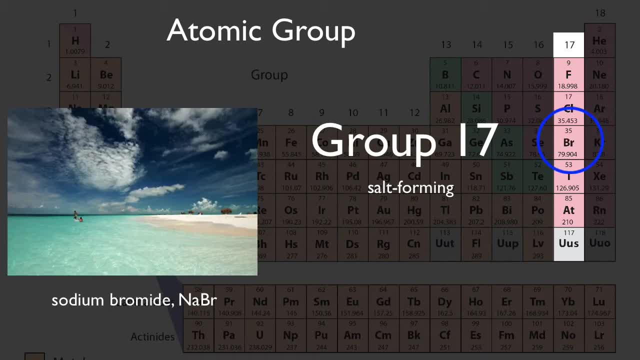 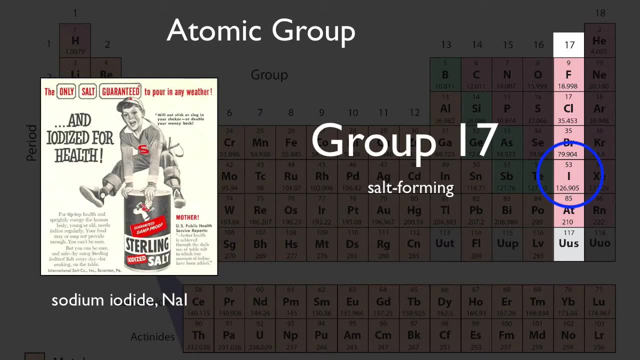 chloride found in table salt. There's sodium bromide- You'll find plenty of that in our oceans- And sodium iodide, which is what they add to iodine- Iodized table salt. You see, the small amount of iodine helps prevent a medical condition called. 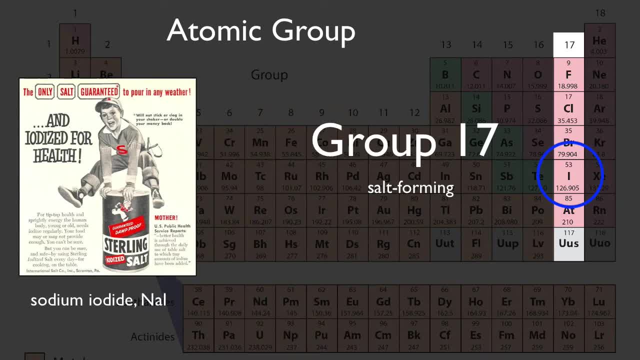 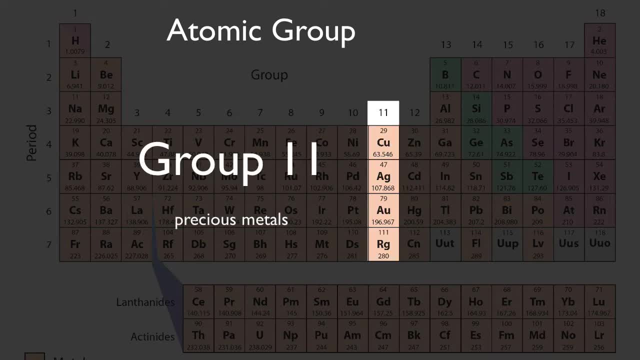 goiter, which is a growth in the thyroid gland. So, elements above and below one another, they share similar properties. Take note of group 11.. This is where you'll find the precious metals gold, silver and copper. So it's no coincidence that they appear directly above and below each. 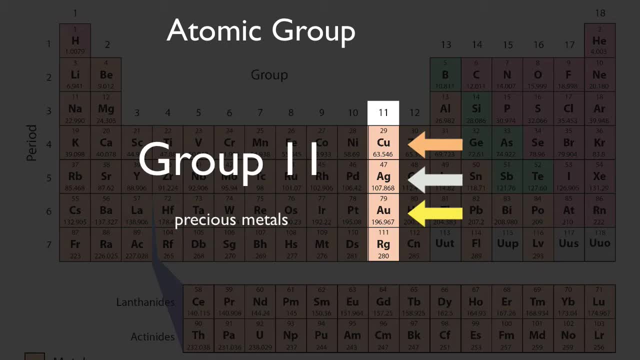 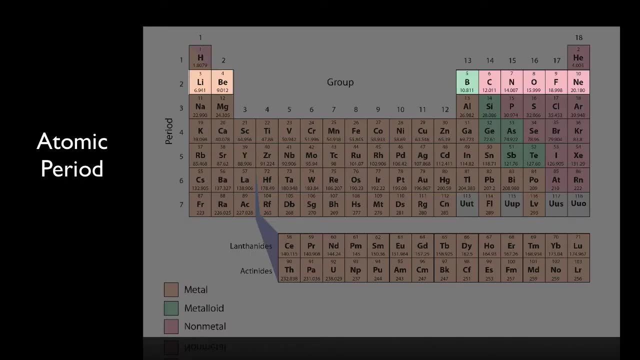 other. in the periodic table We say they're in the same atomic group or family. A horizontal row is called an atomic period. Across the horizontal row there's a gradual change in some property of the elements. The one I like to talk about most is 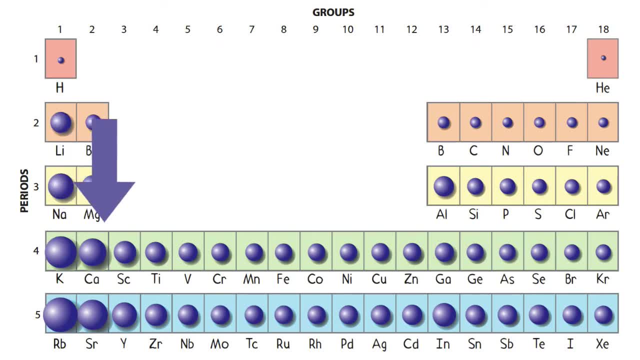 atomic size. Atoms to the left tend to be larger than atoms toward the right. We call this a periodic trend, and it works up and down vertical columns too. Atoms at the bottom of a group tend to be larger. Putting it all together, we see that atoms at the bottom of a group tend to be larger. 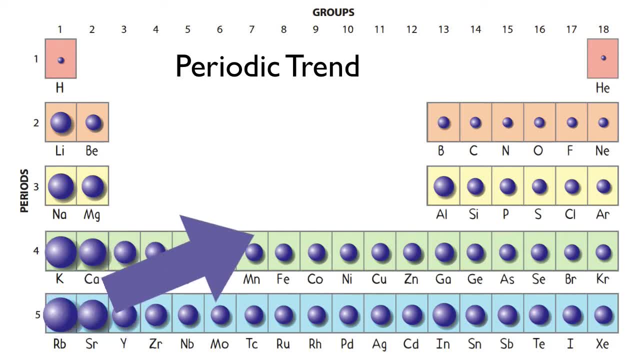 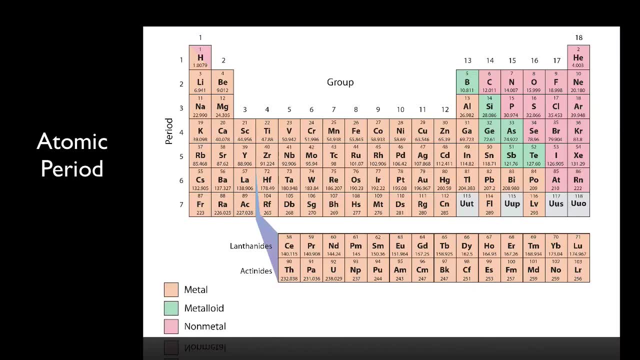 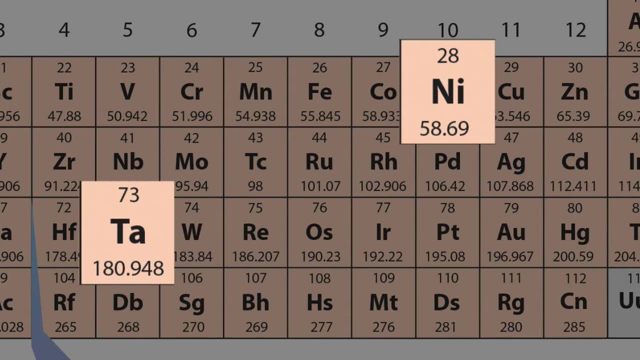 Those of elements to the lower left of the periodic table. they're the largest atoms. Those to the upper right, they're the smallest. So let's do a test: Which is larger, A nickel atom or a tantalum atom? Look, there's no need to memorize anything, Just look, You'll see. nickel is closer to the. 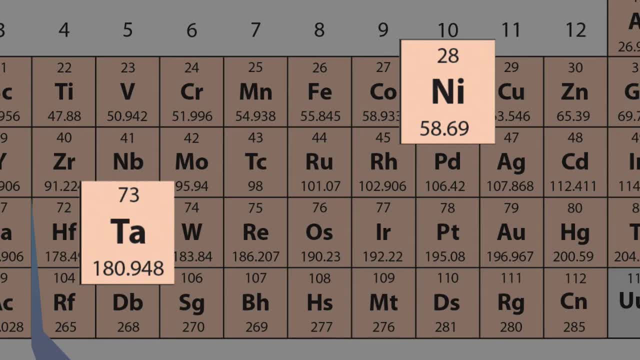 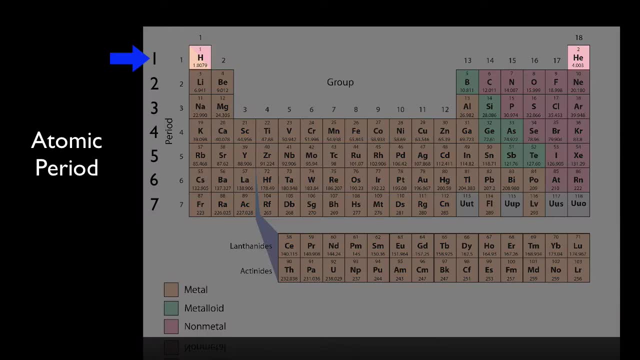 upper right. so it's likely the smaller of the two, And it is. There are seven periods. Notice. the first period only has two elements: hydrogen and helium. The second period has eight elements: lithium through neon. There are also eight elements. 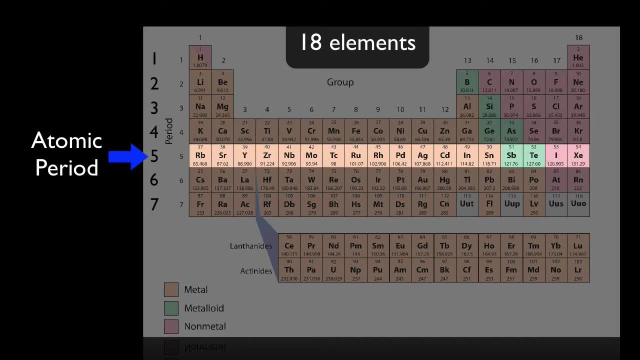 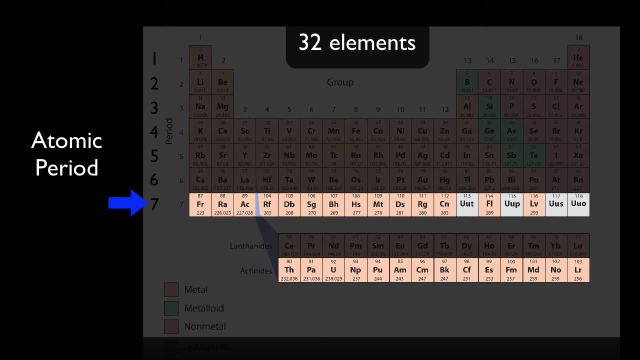 yeah, in the third period, The fourth and fifth periods, well, they each have 18 elements, while the sixth and seventh periods each have 32.. Well, it's theorized that the seventh period should have 32.. It's just that not all of them have yet been discovered. 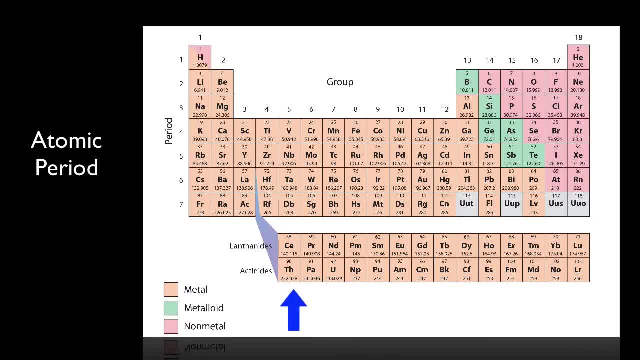 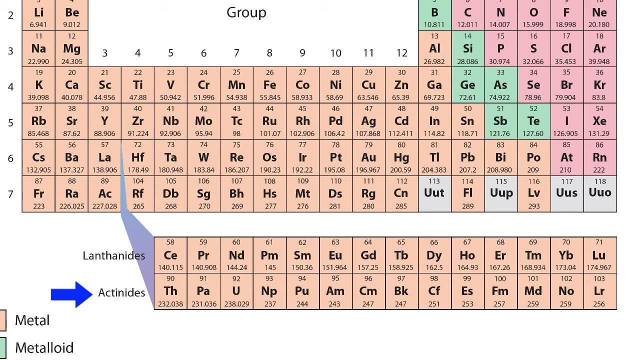 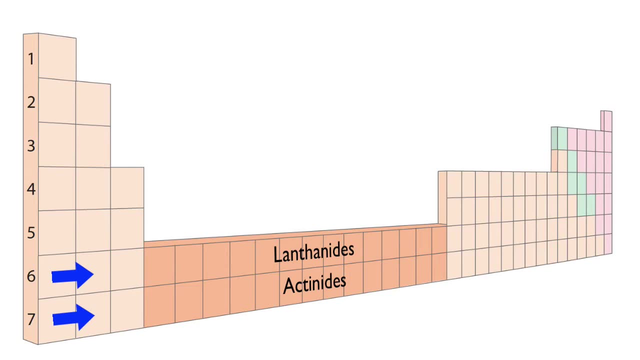 What's this lower box all about? These are the lanthanides and actinides. They are, if you will, subsets of the sixth and seventh periods. Technically they should be squeezed into these periods like this, But then the periodic table doesn't fit very well within a regular 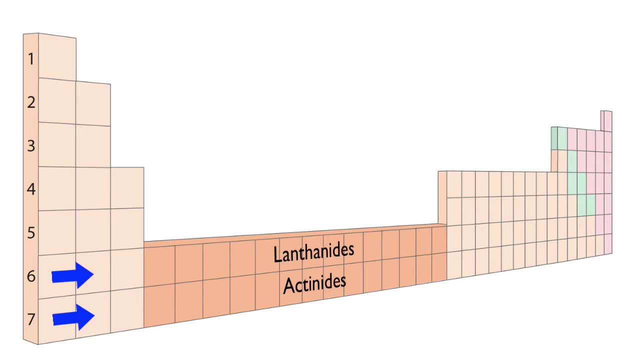 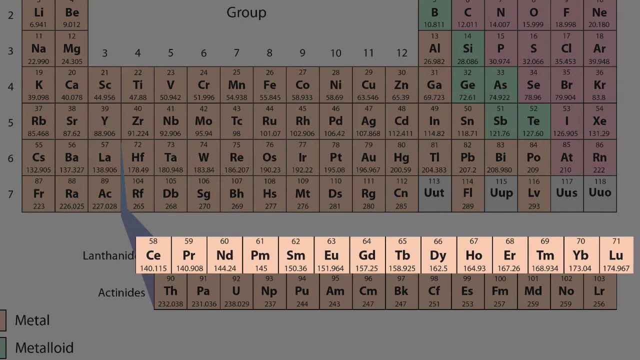 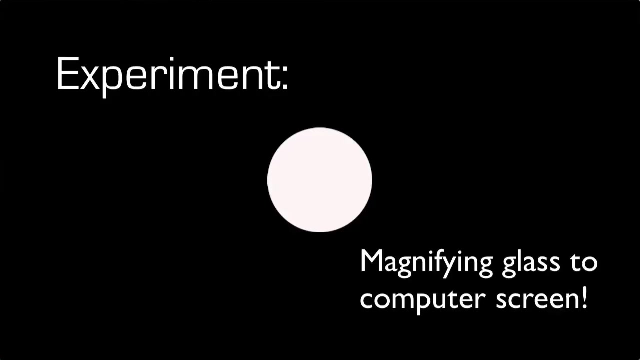 sheet of paper or your computer screen. That's why they're drawn below the main body of the periodic table, The sixth period, lanthanides. they're fascinating, In fact. I can show you some in action right now. Are you looking at an LED, digital screen? Well, the colors you see are being generated by 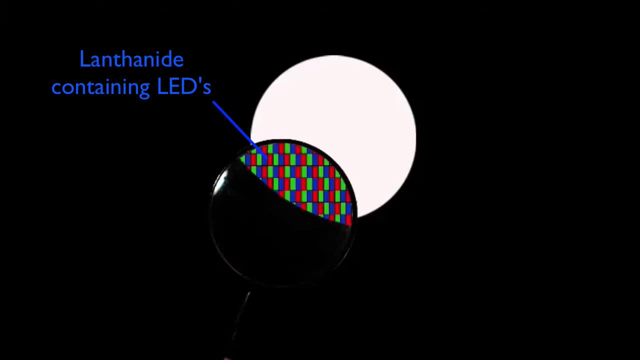 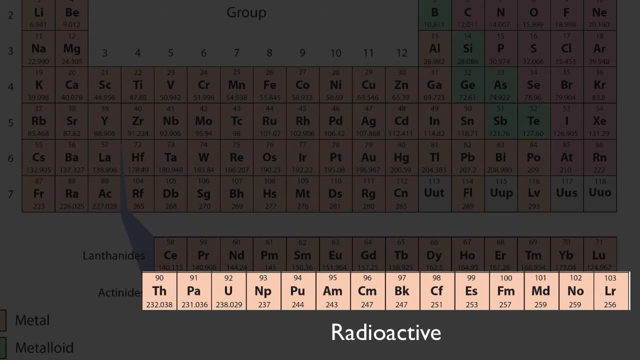 lanthanides within the LED. Huh, The actinides are all radioactive elements. Later we'll be discussing the concept of radioactivity and also nuclear energy, But right now I should tell you, most nuclear energy is generated by the fission of isotopes of uranium. 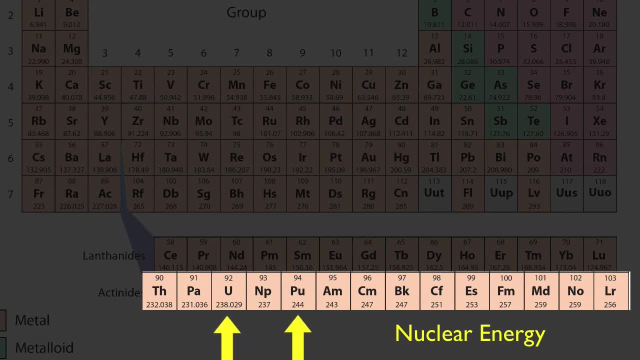 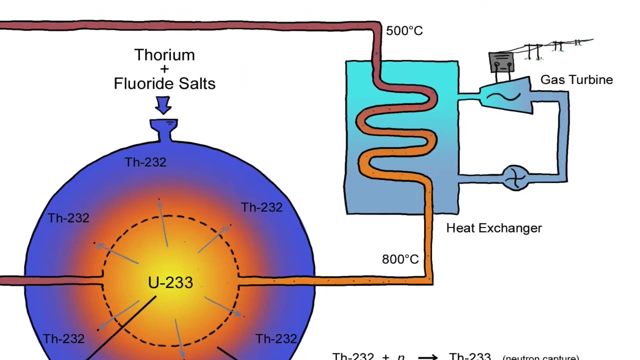 and plutonium Here. these are actinides, But there's much promise in the first actinide, which is thorium. You really need to learn about thorium nuclear reactors. They offer a much more efficient, safe and environmentally friendly means of nuclear energy. We'll discuss thorium. 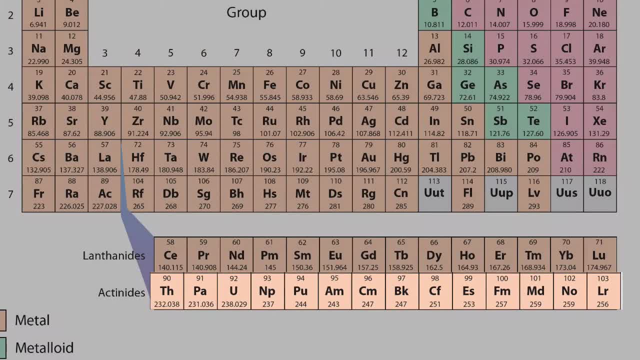 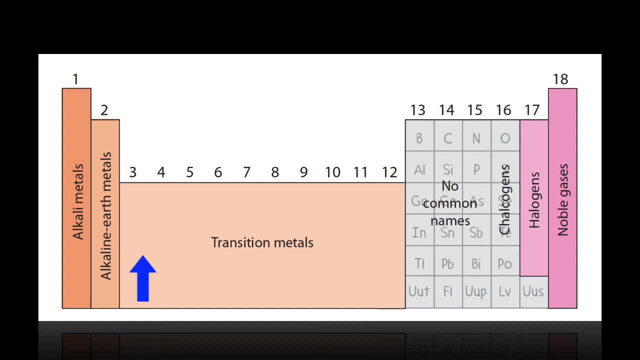 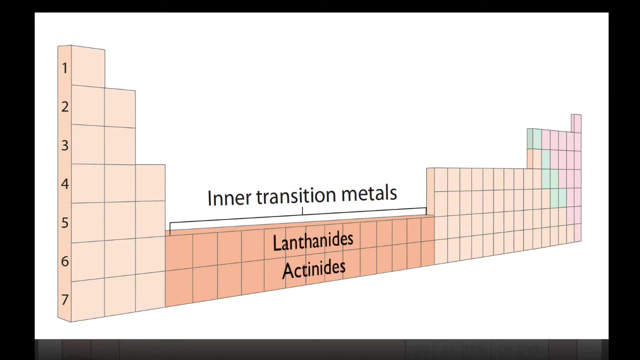 reactors later. I should mention how blocks of elements have traditional names, as shown here: The transition metals, for example. they transition from one side of the periodic table to the other, The lanthanides and actinides. they're collectively called the inner transition metals. Now I'm 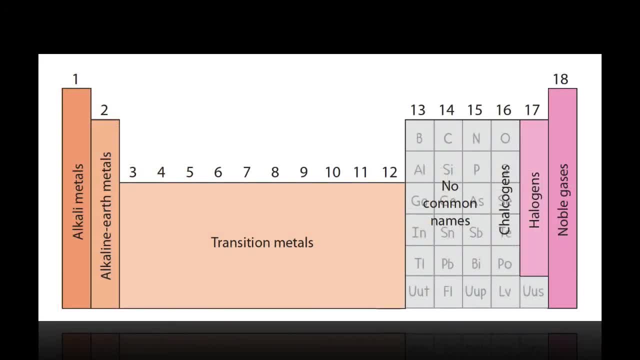 confident. your instructor won't ask you to memorize the periodic table, but he or she may want you to become familiar with the names of these blocks. Why? For communication. That way you won't get lost if someone ever asks you what's your. 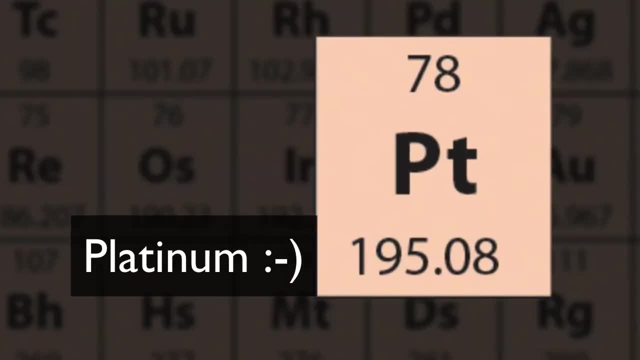 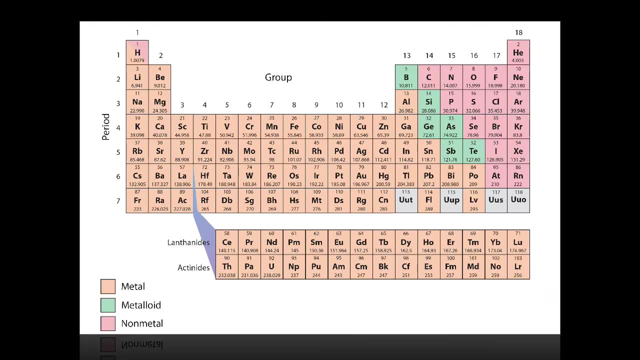 favorite transition metal. For now, the task at hand is becoming familiar with the basic organization of the periodic table. Please don't spend your valuable time and energy memorizing this chart of the elements. Instead, focus on its remarkable organization. I should 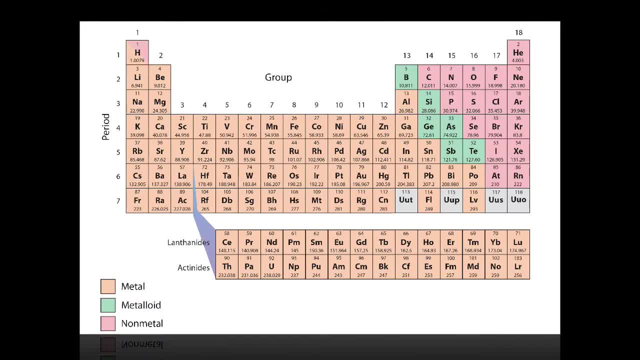 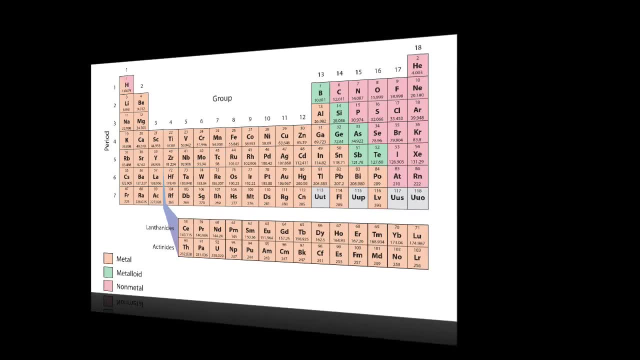 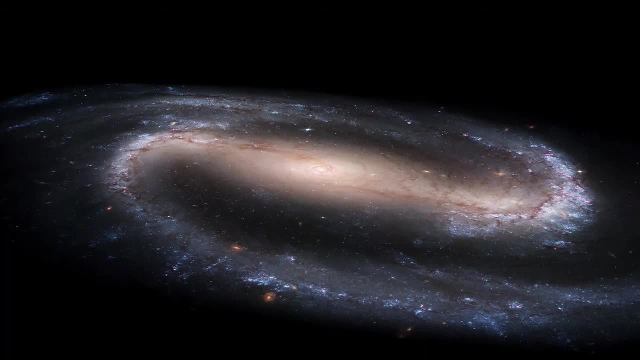 underscore. the periodic table is nothing we humans invented. Rather, it's a natural organization of the elements that we discovered. You know you could travel to a distant civilization in a distant galaxy, and you'll likely find a similar organization of the elements posted on the walls of their chemistry classes. Think. 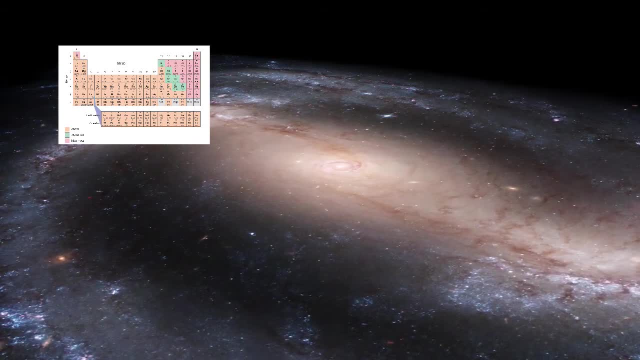 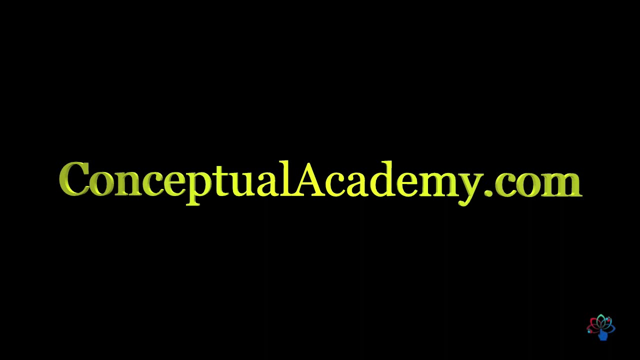 about that And good chemistry to you. Subtitles by the Amaraorg community. 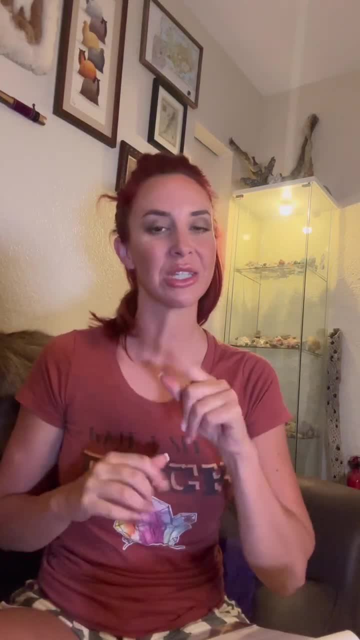 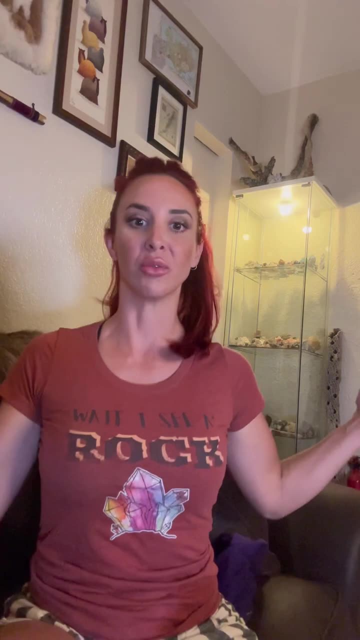 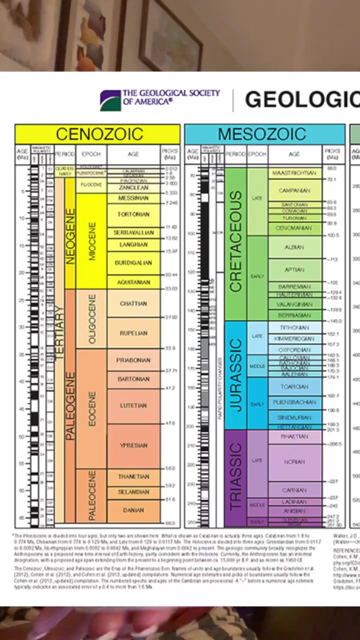 Hey everybody and welcome to day three of my short series, geology 101.. Today we're talking about geologic time, or the geologic time scale. Now, geologic time, what is it? It's also known as a geologic time scale, this guy, and it's a representation of time based on the rock record. 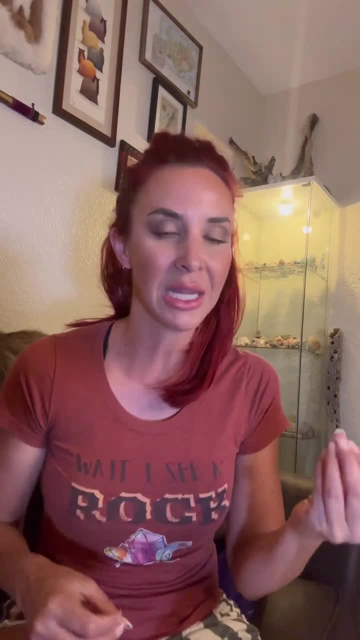 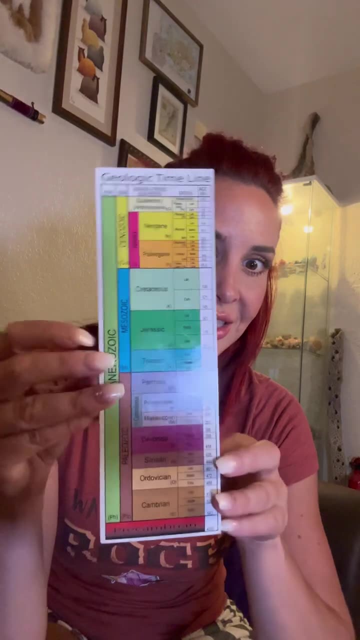 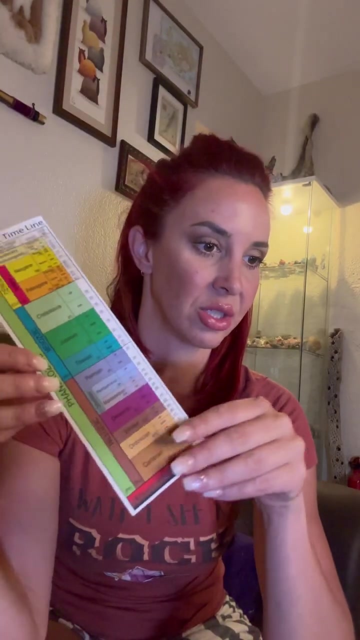 on earth. Geoscientists use this to describe timing and relationship of events in geologic history. It's quite well known, it's quite used. This is one of my original bookmarks of the geologic time scale. Came from my college. Either I'm a hoarder or sentimental, or just made a really. 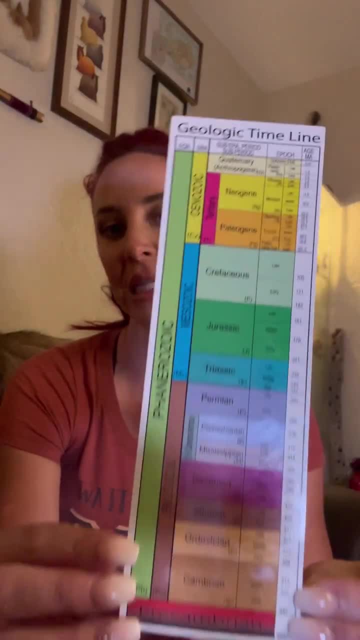 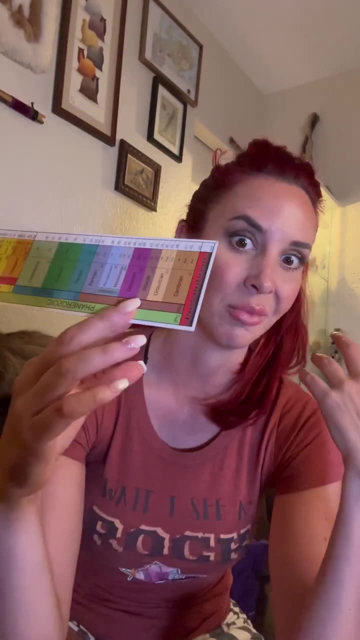 good bookmark One or the other. I had to memorize each one of these things. Basically it was a giant brain dump and I put it down on a piece of paper and I hoped I was correct and I passed. So you know, must have been a little bit correct, But it's a very good thing to have in your back pocket.